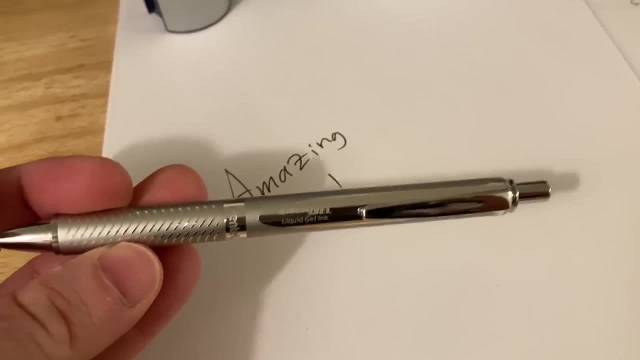 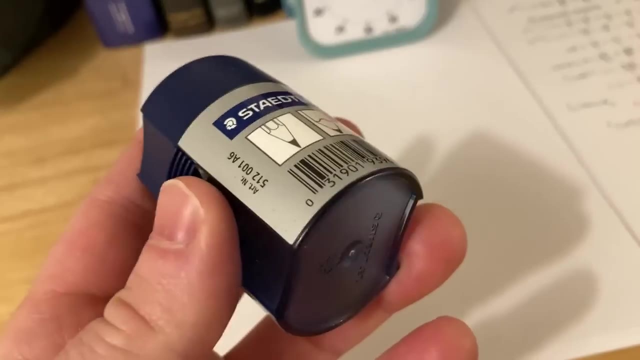 but if you're a pen person, this one's pretty incredible, Although it is a little bit pricey. Of course, everyone needs a sharpener, and I like having one. that's pretty good. This one doesn't use batteries, so I can take it with me, So if 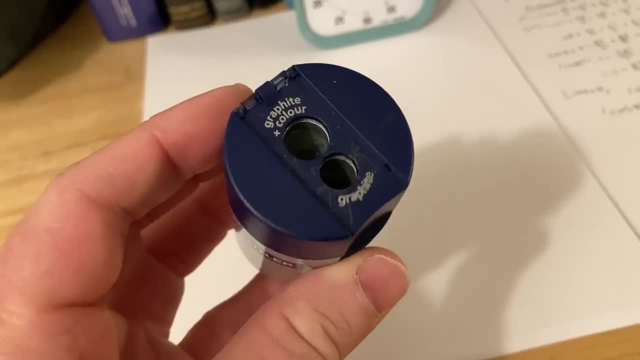 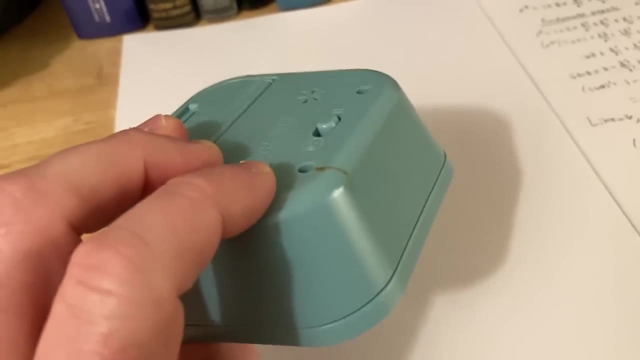 I decide to do math outside. I can take it outside, and it doesn't require any electricity or anything like that. One of the most important components is, of course, a timer, So you can use this to time your sessions, which I highly recommend. This is a really simple. 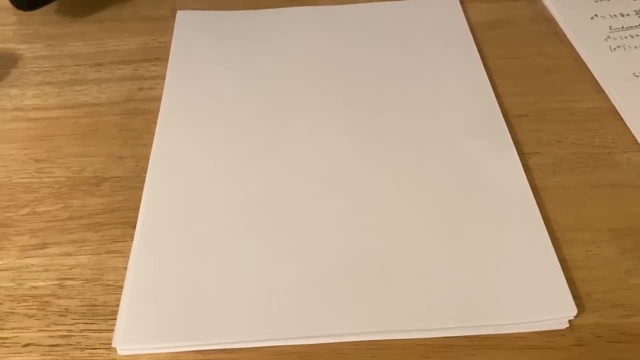 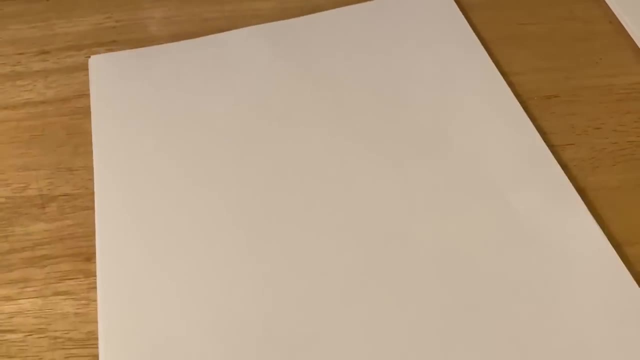 one that works great and it uses one AA battery. Of course, you can't do math unless you have something to write on, and this is paper. Notice: this paper doesn't have lines. The reason I use paper with no lines is because 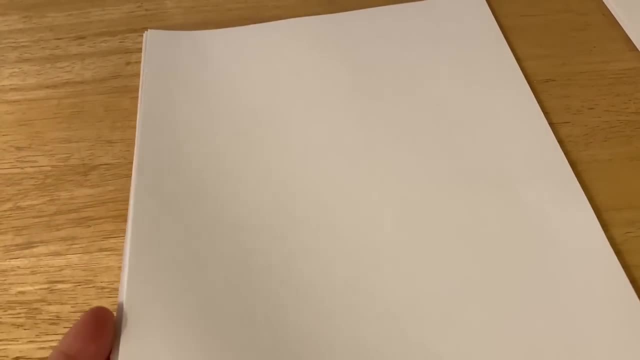 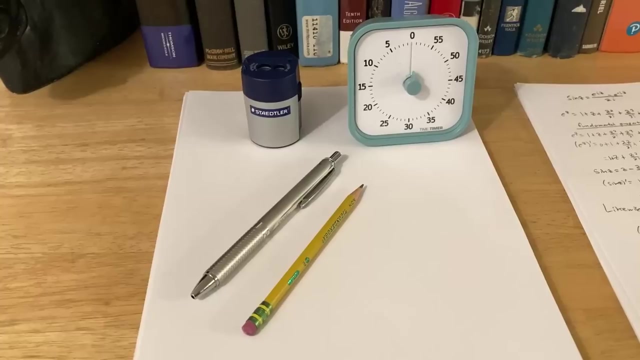 the smartest person I ever met used paper with no lines and I thought maybe that's making him better at math. So I started using paper with no lines and ever since then I have been hooked. So you've gathered your supplies. You have either a pen or pencil, a timer, a sharpener. 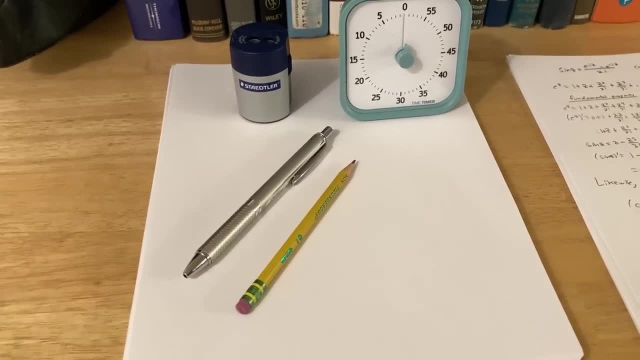 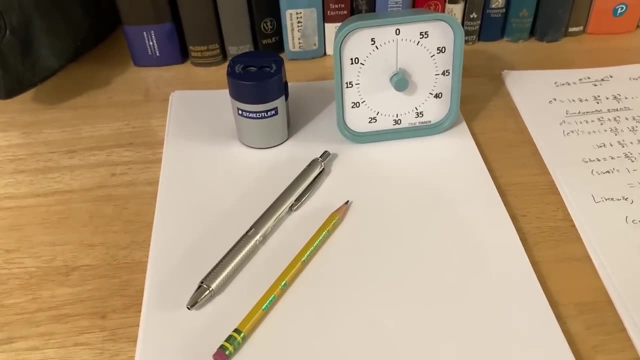 and some paper that you're comfortable with, And it doesn't have to be these. I would just recommend using what you prefer. If you prefer a mechanical pencil, get that. Remember. you want to be as comfortable as possible when you're working on math. 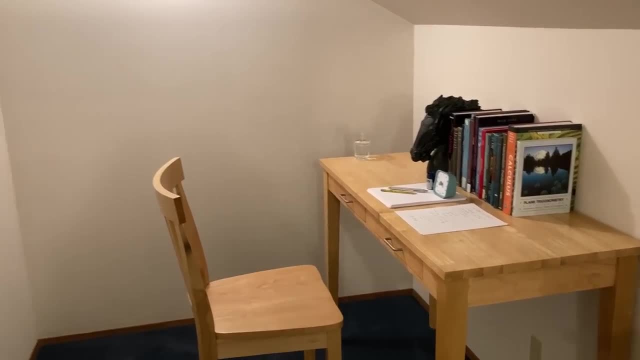 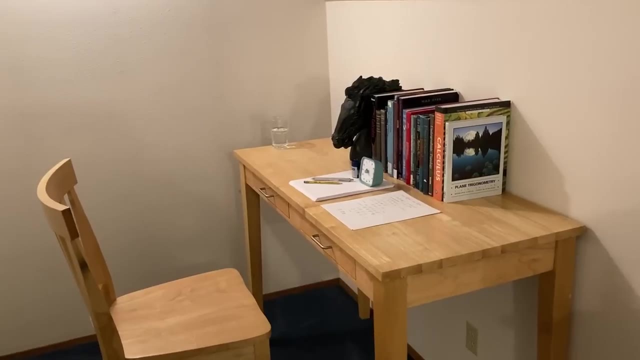 The next thing you want to do is pick a quiet location. You can see here, the room that I'm actually in is very, very small and very secluded and it is extremely quiet. So try to find the quietest spot you can so that you can sit down and be productive. If you can't find 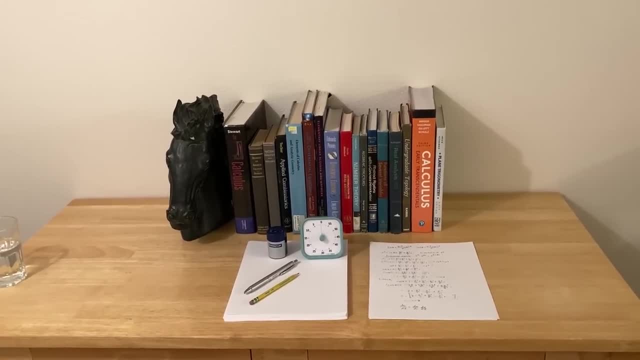 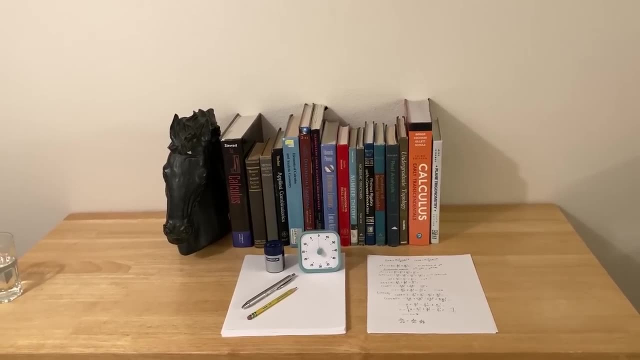 a quiet location to study, then try to find a place where you can go that is a little bit more quiet. Consider college libraries or even public libraries. Those are usually pretty good places to go study. The next step is a really fun step and it's picking a book, And this is a step that you 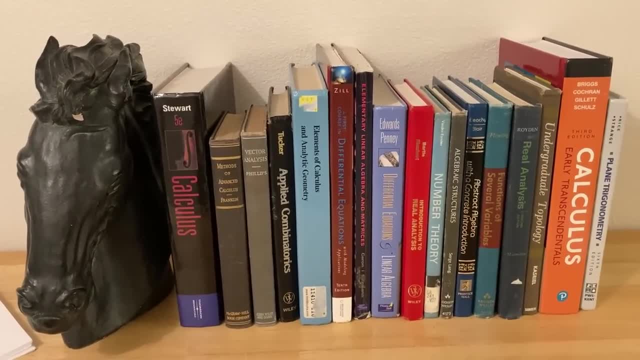 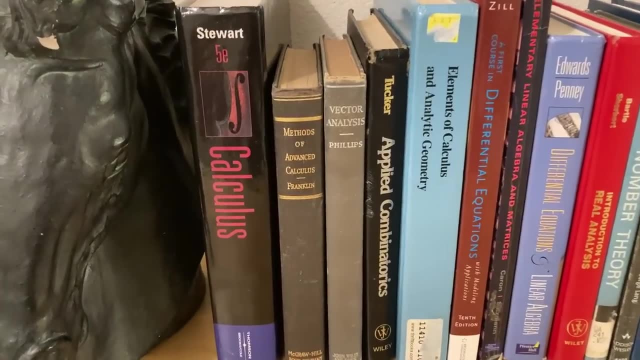 might get stuck on. My advice is: just pick a book and go with it. If you can't make a decision, just grab one of your math books and start reading it. Now, I've got a lot of books here, as you can see. We've got some calculus, advanced calculus. 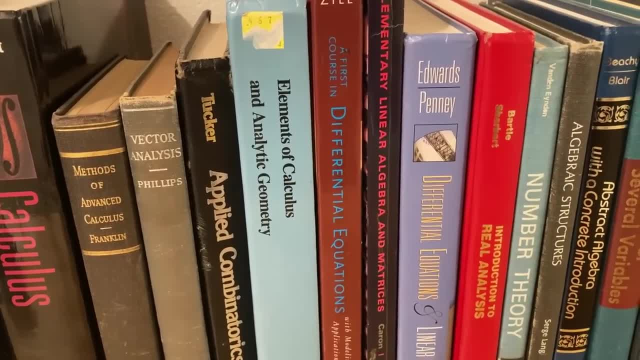 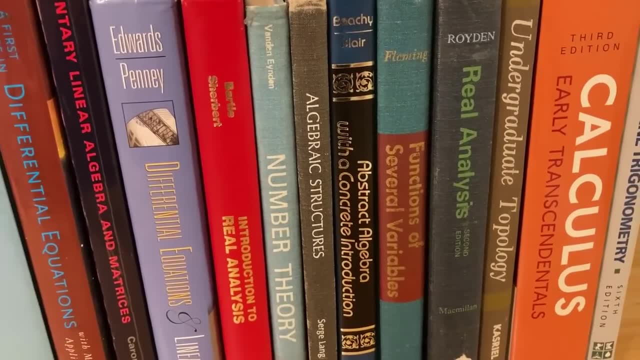 vector analysis, combinatorics, more calculus, differential equations, linear algebra, more differential equations, real analysis, number theory, some abstract algebra, some multivariable calculus, some real analysis, some topology, a little bit more calculus and some trig. 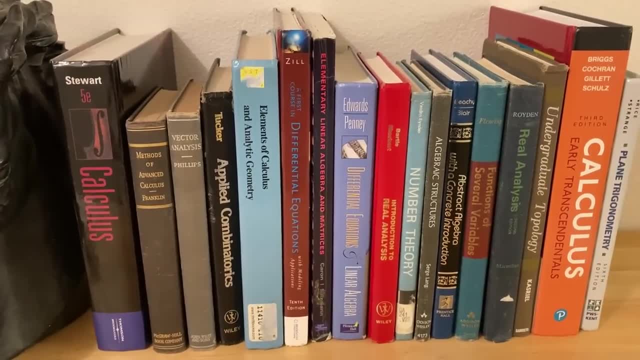 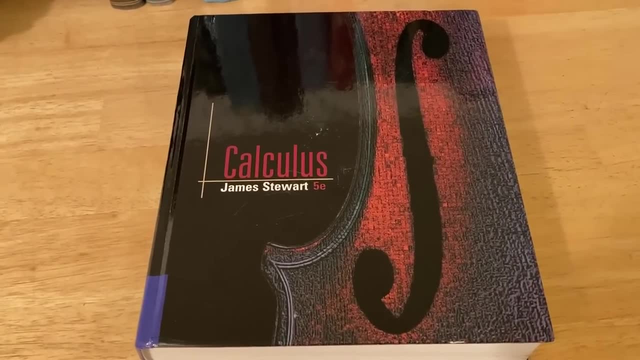 So all kinds of choices And for the purposes of this video, I'm actually going to pick one of these books and I'm going to show you how to study, Because this is such a popular book and it is so widely available and it is so widely. 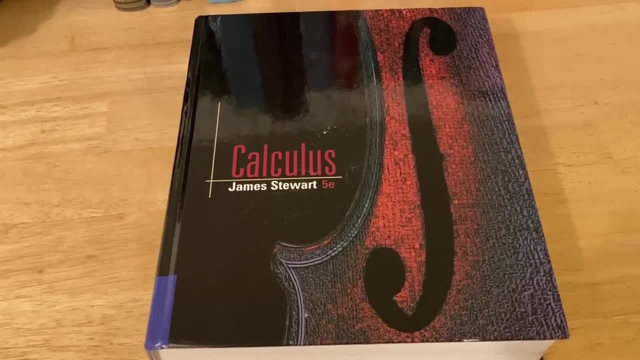 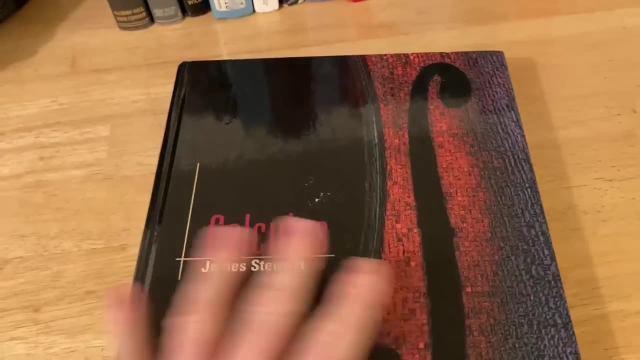 used by colleges and universities all over the world. I've chosen this one. This one is Calculus by James Stewart, and it is the fifth edition. This is a super thick book that people use to take Calculus 1,, 2, and 3 in college. 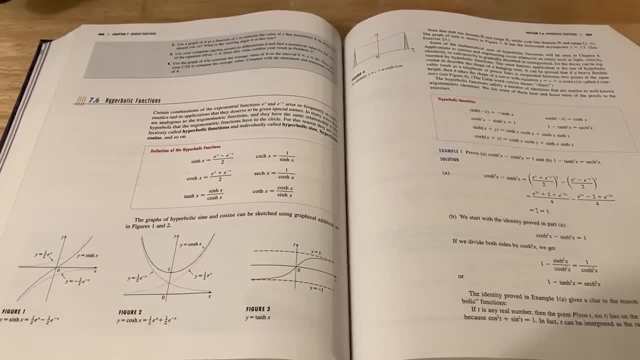 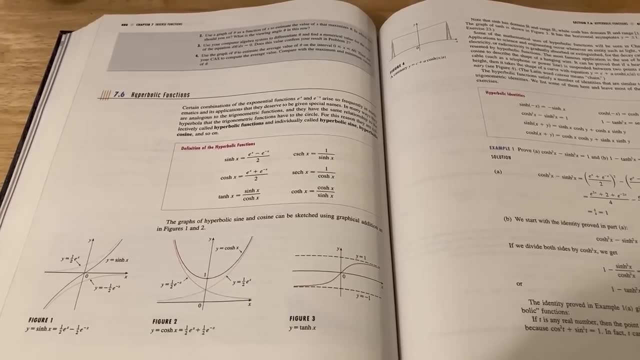 It lists all kinds of languages in the US and in Canada. Once you have the book, you have to decide what section you want to read. My advice is to pick something that you want to read, so something that is interesting to you. but 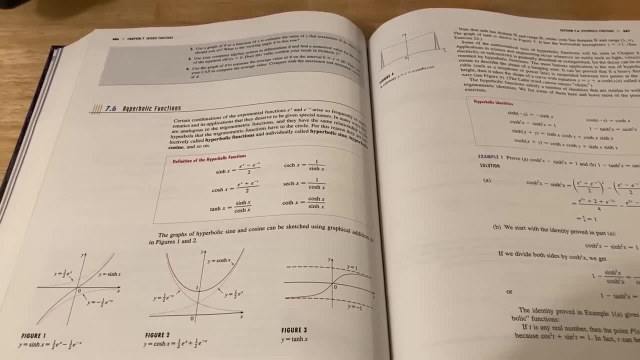 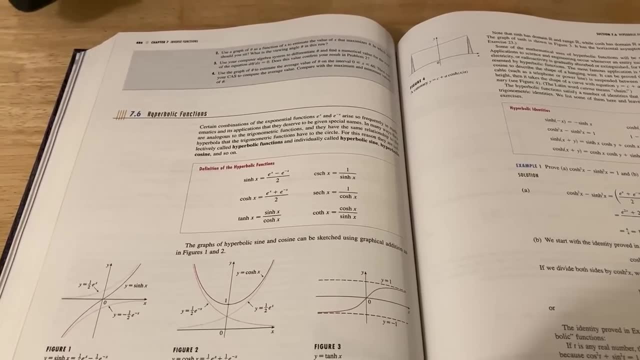 at the same time, you want to pick something that is going to push you a little bit. You want to study something that you really haven't seen before, or something that you feel uncomfortable with. You want to push yourself into that uncomfortable place so that learning actually 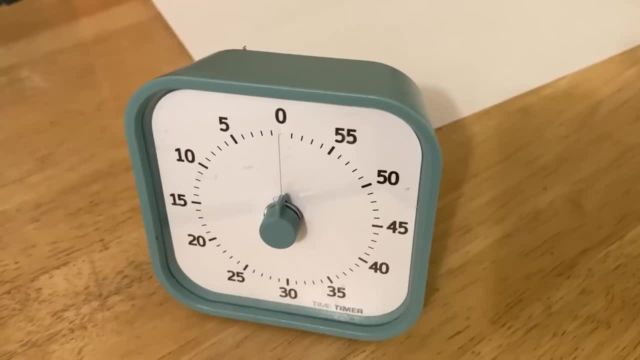 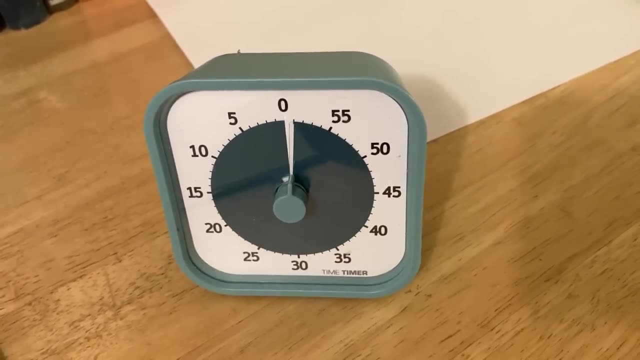 takes place. After all, the whole point is to actually learn something. to set the timer, I like to set it for one hour. I feel like one hour is a good amount of time to study most subjects, And then you just get started. 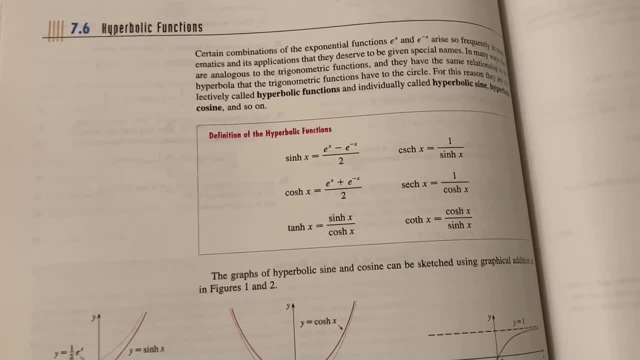 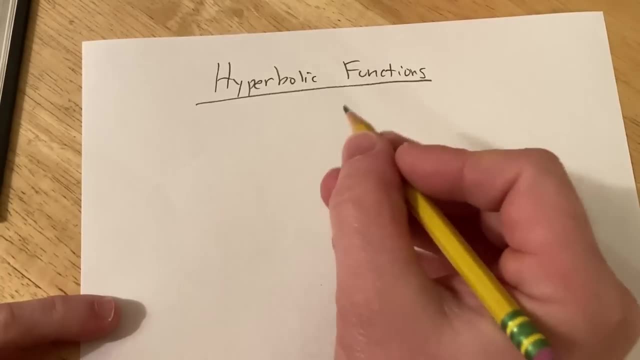 So you start reading the book, You notice that it gives you the definition of the hyperbolic functions. So the first thing you want to do is make sure you know that definition. So how do you do that? Well, the best way to do that is to actually write down the definition. 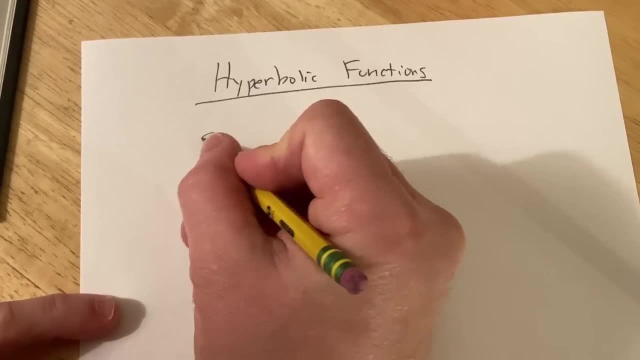 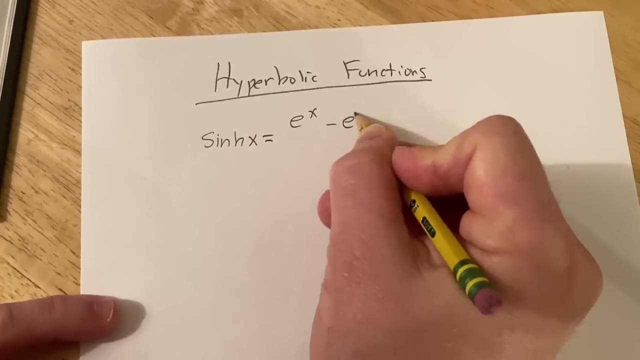 And you want to be able to write it down without looking at the book. For example, the hyperbolic sine of x or sinh x is going to be half the difference of e to the x and e to the negative x. So you take e to the x, you subtract e to the negative x and you divide by two. 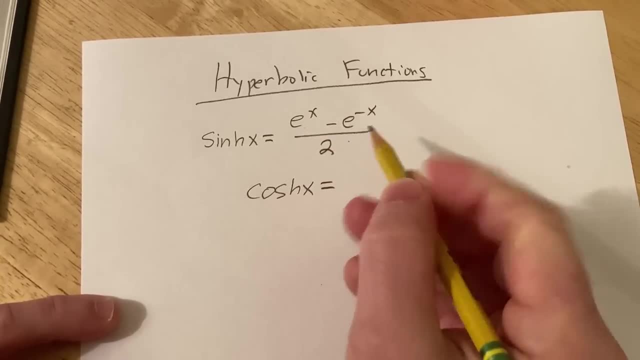 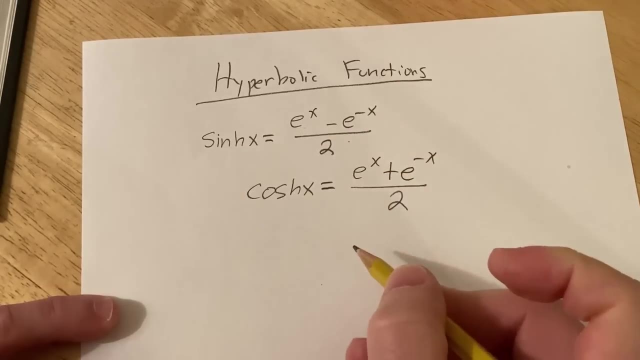 The hyperbolic cosine is going to be the average of e to the x and e to the negative x. So you take e to the x, you add e to the negative x and you divide by two. And for the rest of them, if you notice in the formulas, they're very similar to the trig functions. So you 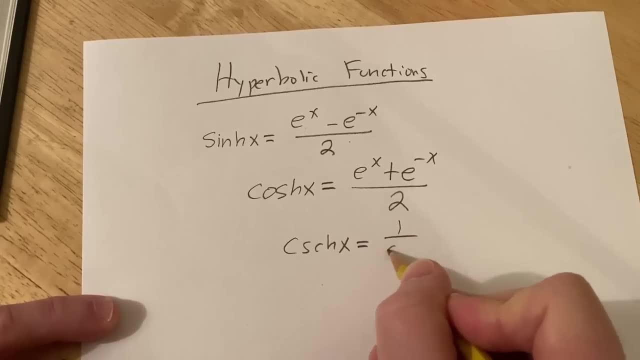 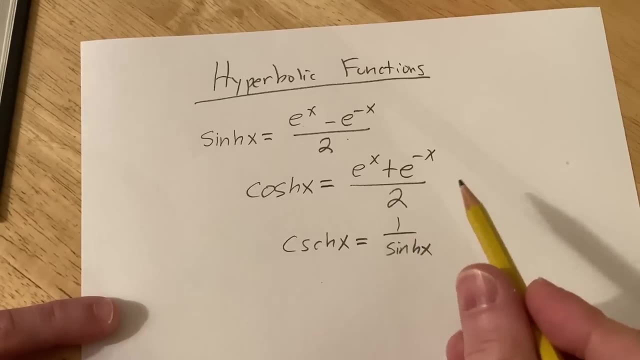 can go on from there and fill in the rest of the formulas For your hyperbolic functions. if you find yourself having to look at the book, you want to start over and do everything without looking at the book until you know the definition's. 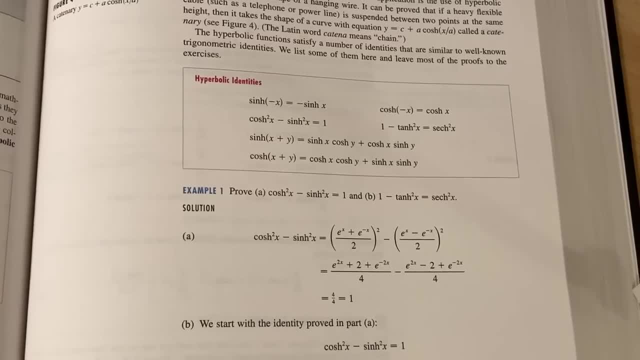 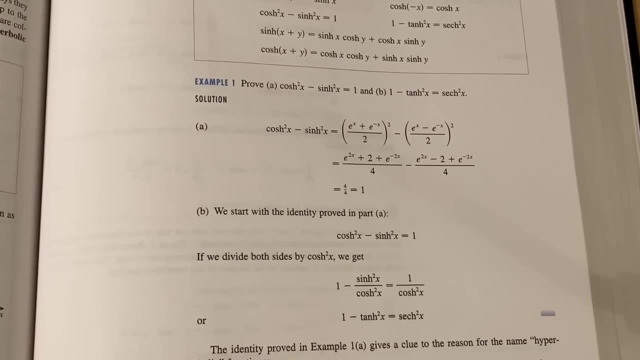 cold As you continue reading the text. you want to work through all of the examples. For example, here you notice they give you the hyperbolic identities and they have a proof of one of them. So maybe prove the one they do, but do it on your own without looking. 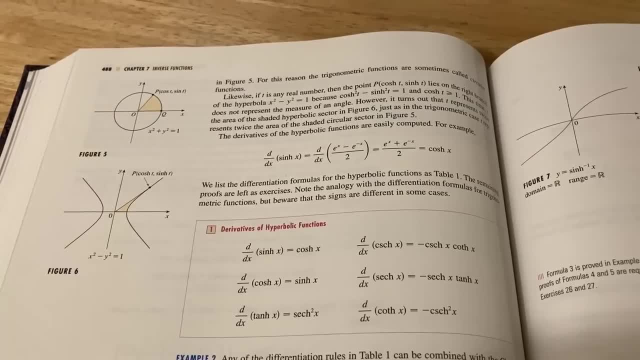 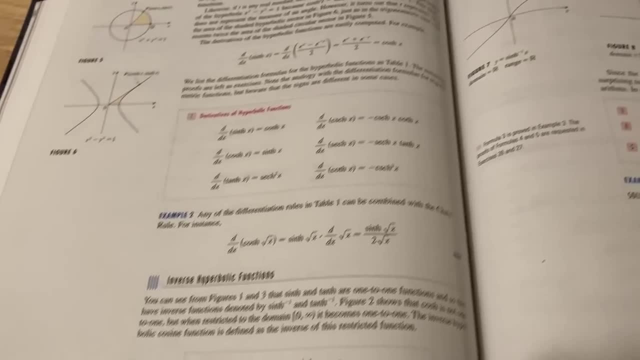 at their solution and maybe do a couple more, just for practice. Then you continue reading the text and doing all of the examples that you can. Not everything will make sense, and that's normal, And you want to just work through it and try to understand as much as. 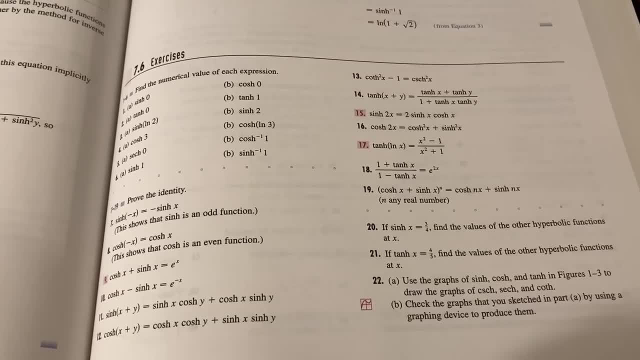 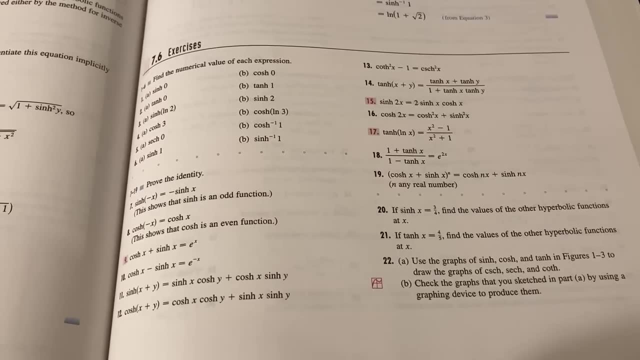 you can from the examples that are given in the book. Once you get to the exercises, you should feel pretty good about yourself, because you made it through the entire section. At this point you should start doing as many problems as you can. In a book like this, you'll have answers to most of the odd-numbered problems. 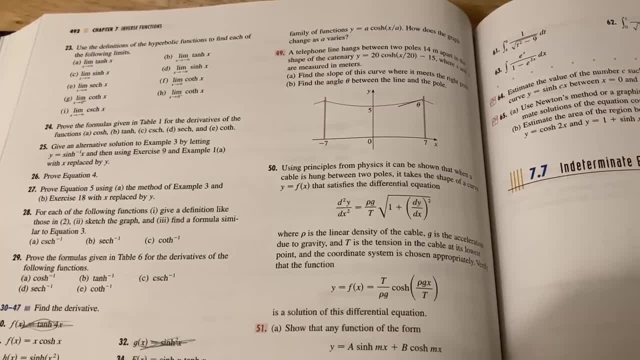 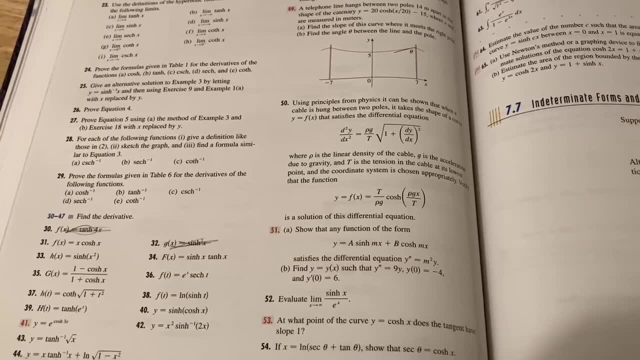 which really helps. One thing you will notice in most math books is when you get to the problems at the end of a section, you're going to find problems for which there are no examples in the book. So you wonder: how am I supposed to figure those out? Well, that's when you have to go. 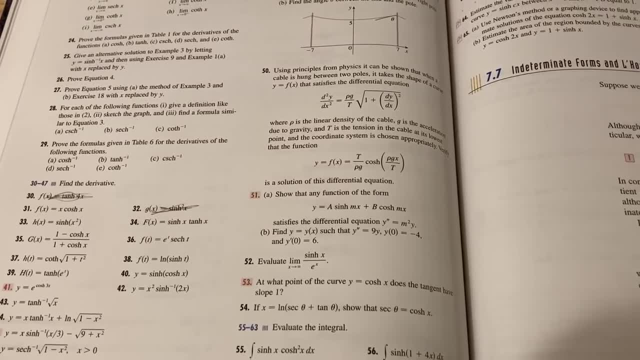 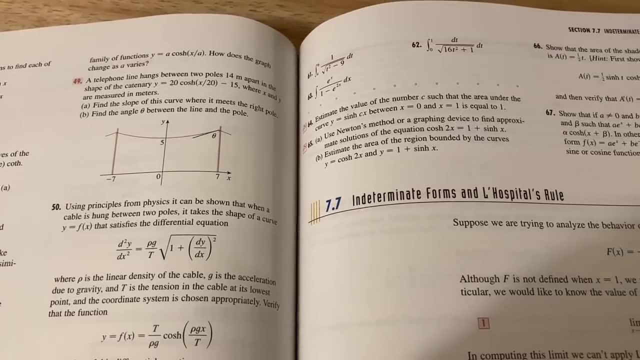 back to the section and try to find information that you can use to help you solve those problems. If you still can't figure them out, it's okay. Books like this have tons of problems and some of them are harder than others. And if you're wondering why the author didn't include 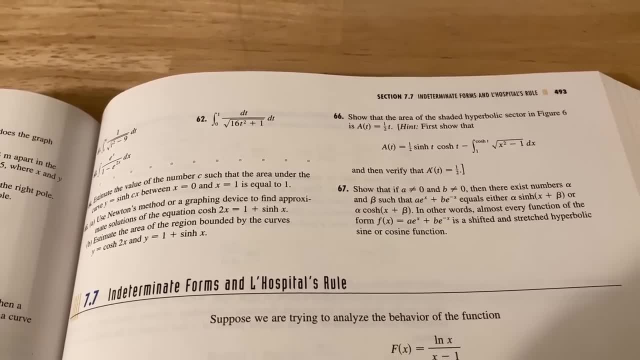 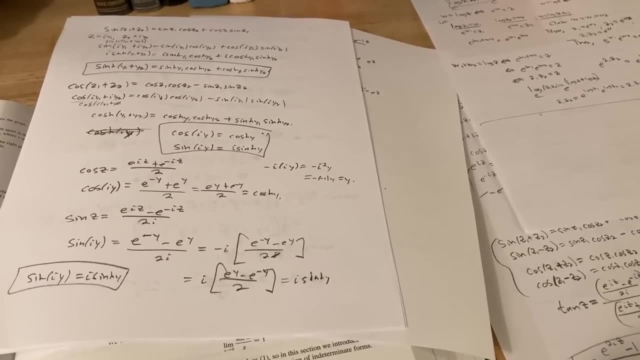 examples of every single type in the book. it's because then the book would be insanely huge, So they have to pick and choose what content they present in the book. So now you're done studying, You should feel good about yourself. You got a lot done And 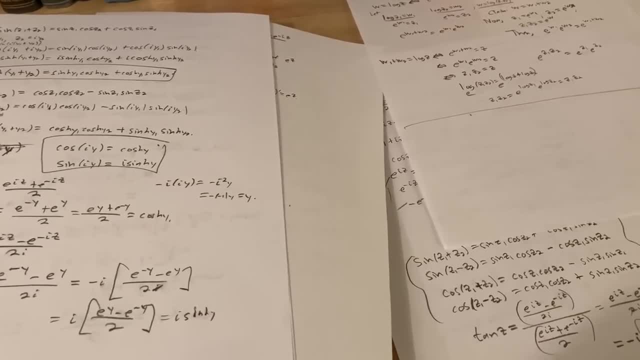 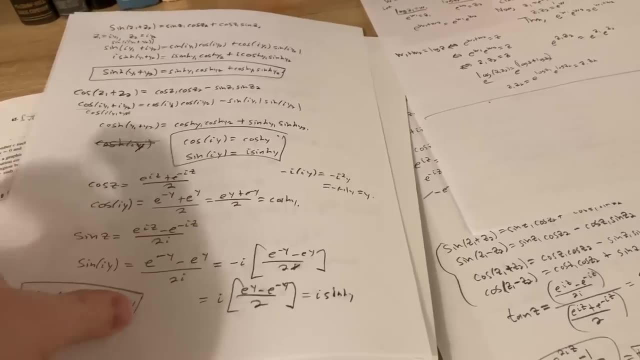 this is the last step. It's to reflect, Reflect on what you did, Reflect on how meaningful your time was. You just took an hour of your life and you learned a lot of mathematics. If you like, you can keep your work. You can buy a hole puncher and put it in a binder. 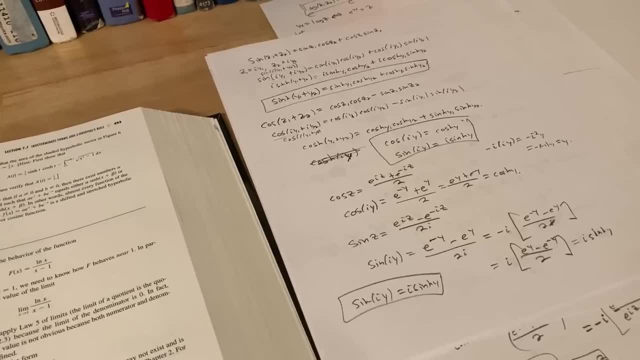 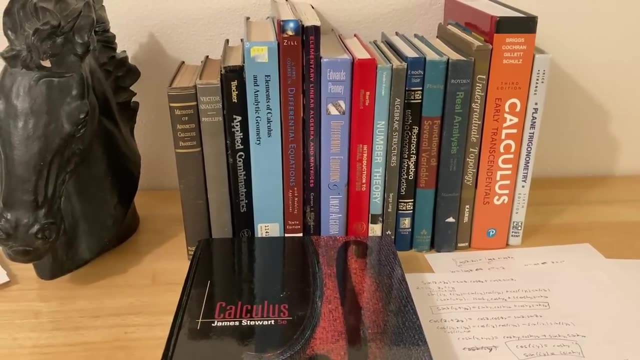 You can stack it up in a big stack Or you can throw it away. Whatever you like. As the day proceeds, you're going to find yourself thinking about some of the math you did. Maybe there were some points that you found confusing And you might feel a little. 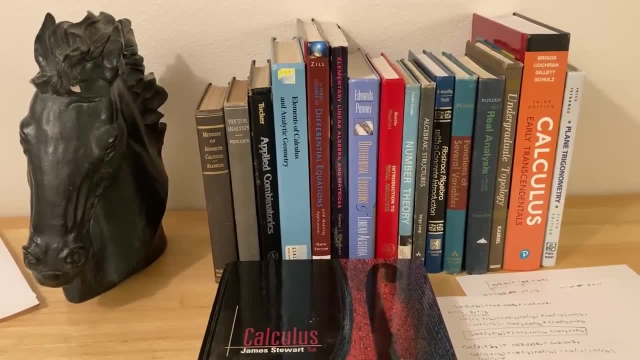 bit confused, And I really think that's normal When you study math and when you read a math book. you're not going to be able to figure out what the math is, You're not going to understand everything, You're going to have moments of confusion. And those moments of 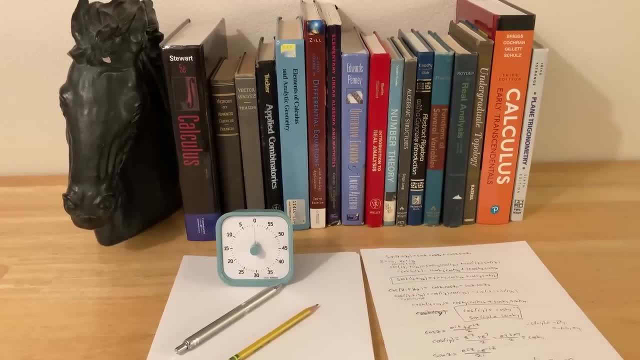 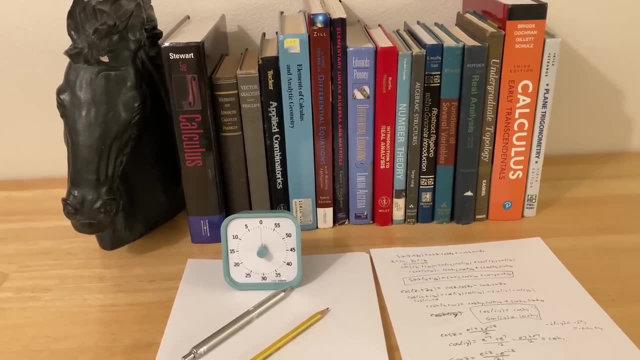 confusion should motivate you to study more next time. One of the great things about self-study is you can study whatever you want. So the next time you have a study session, you can study something completely different. If you didn't like the book that you were using, you can get a different book. Math books are so cheap.